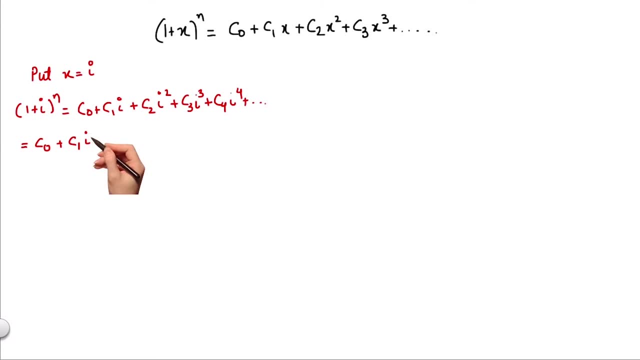 this we would get c0 plus c1, iota minus c2 minus c3, iota plus c4 and so on. Separating the real and imaginary parts, we get c0 minus c2 plus c4, and so on. Alternate plus and minus sign: plus iota, c1 minus c3 plus c5, and so on. 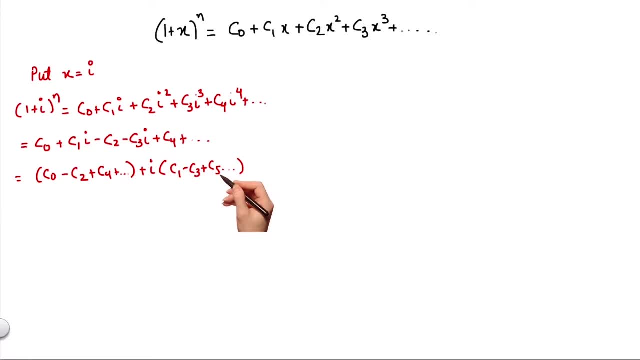 Again, alternate plus and minus signs. Now let's try and put x equal to minus iota and see what happens to this expansion. It would become 1 minus iota whole to the power. n equals c0 plus c1 times minus iota. plus c2 times minus iota whole square plus c3 times minus iota whole. 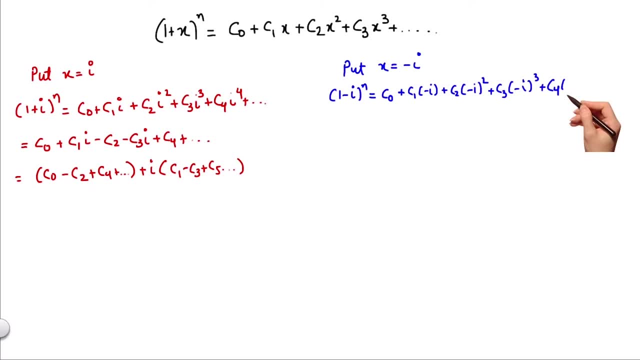 cube plus c4, times minus iota, times whole to the power 4, and so on. Simplifying this, we get c0 minus c1, iota minus c2 plus c3, iota plus c4, and so on. Separating the real and imaginary parts, we get c0 minus c2 plus c4, and so on, minus iota, c1 minus c3 plus c5, and so on. 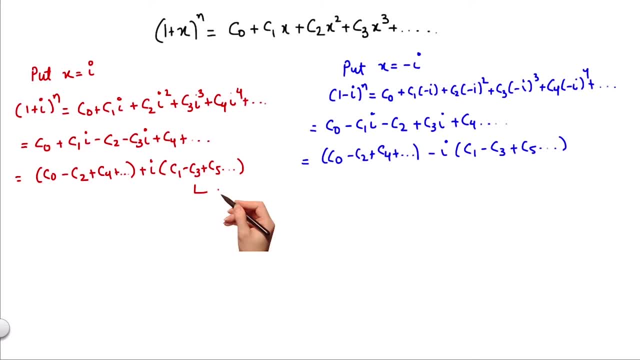 Now, if I were to take this equation as number 1 and this equation as number 2, I would get c0 minus c2 plus c4, and so on. Separating the real and imaginary parts, we get c0 minus c2 and this equation as number 2.. And if I were to calculate 1 plus 2 divided by 2,, 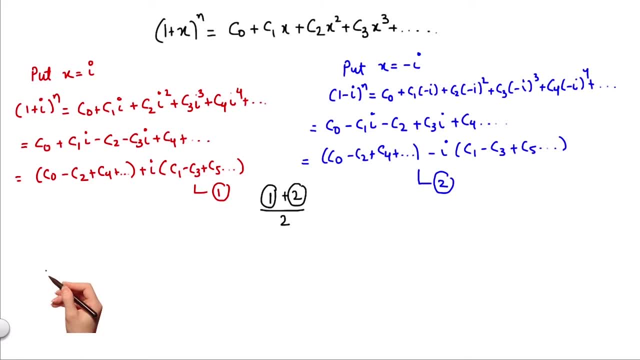 let's see what we get. We would have 1 plus iota to the power n, plus 1 minus iota to the power n, divided by 2 on the left hand side, Whereas the imaginary parts would cancel out and we would have on the right hand side. 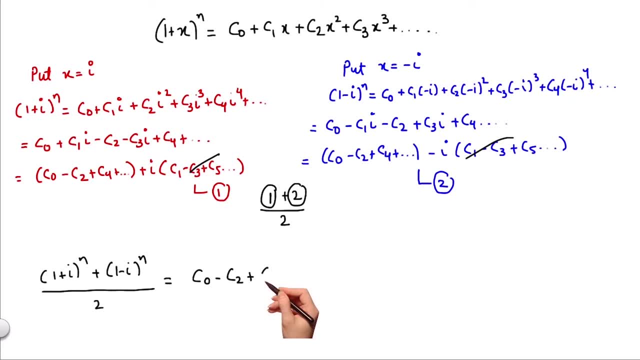 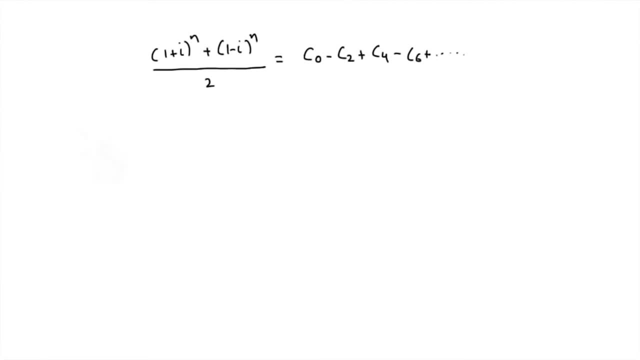 c0 minus c2.. Let's liquidate the imaginary parts. Let's see what we get. We get 1 minus iota to the plus c4 minus c6 and so on. Now we know that we can write 1 plus iota as root, 2 into e to the power iota pi by 4.